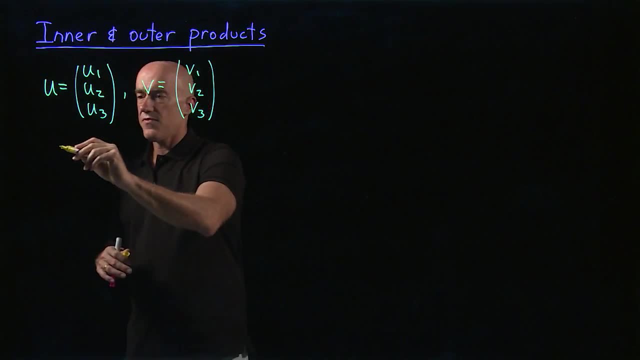 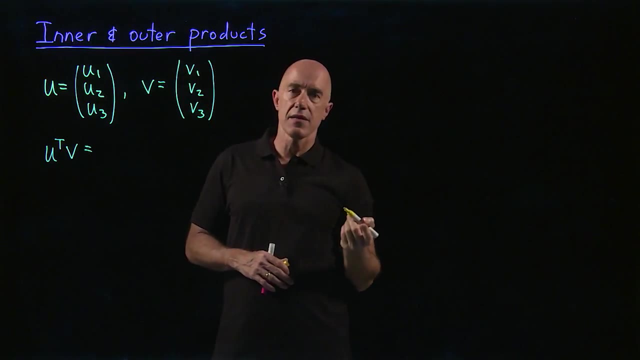 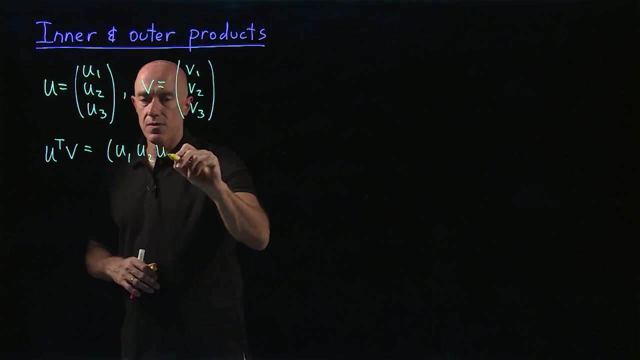 use the transpose operator. So if we write transpose times v, then we'll have u1, v1, v2, v3.. And the transpose of a column vector is a row vector, So we have u1, u2, u3 times. 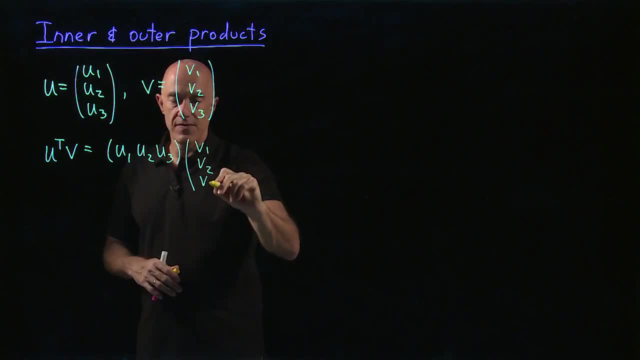 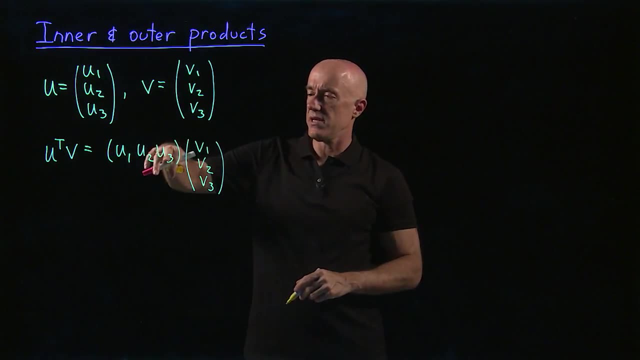 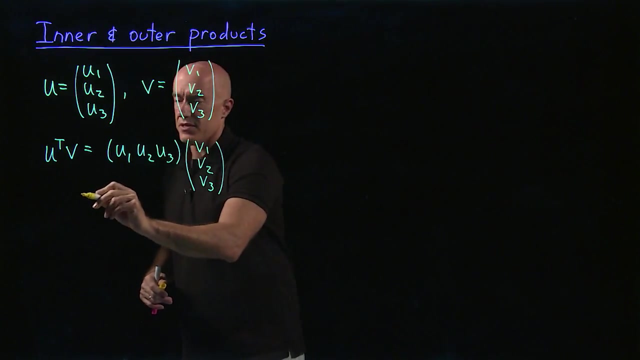 v, which is v1, v2, v3.. So here we have a one row, three columns, So one by three times three by one, and we end up with a one by one, which is what we call a scalar. So this is. 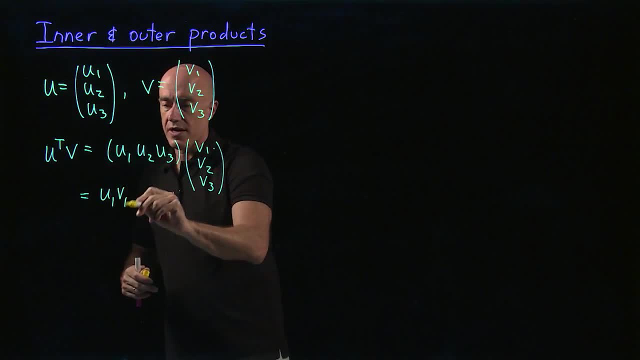 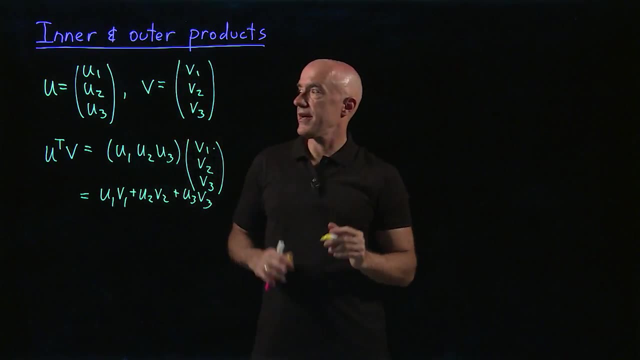 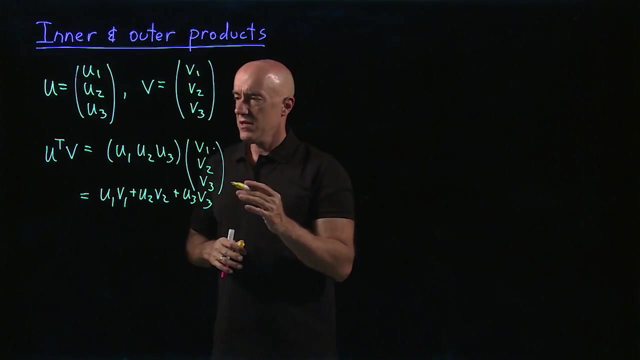 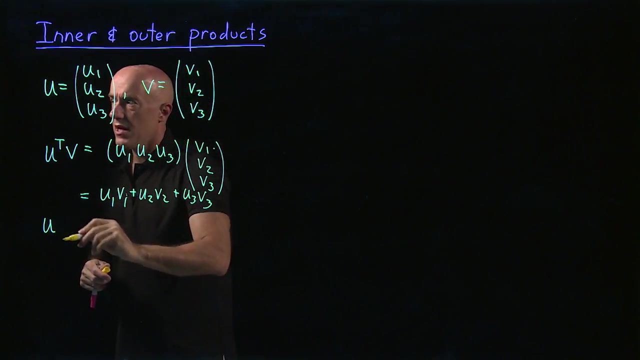 straightforward Multiplication: u1, v1 plus u2, v2 plus u3, v3.. OK, We have some definitions here that are useful. So if this turned out to be zero, so if u and u transpose, v equals zero, then 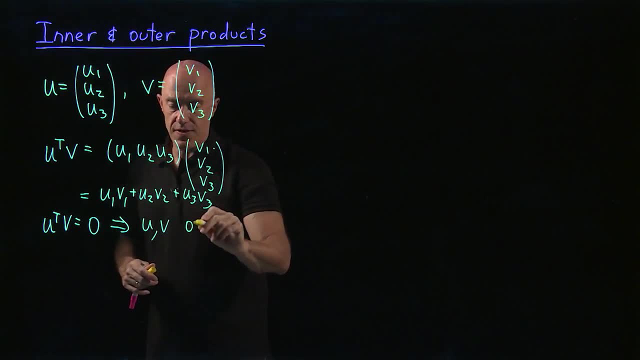 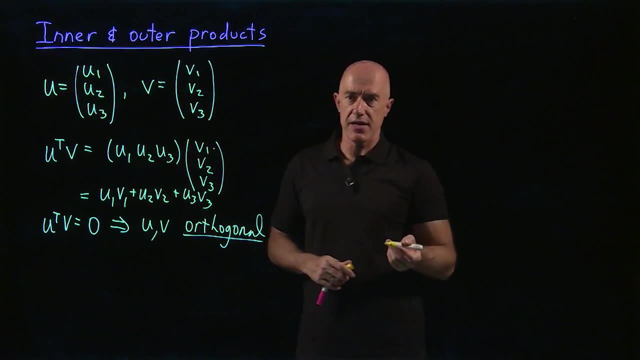 we say that u transpose v equals zero, then we say that u transpose v equals zero. And then we say that u transpose v equals zero, then we say that u transpose v equals zero. u and v are orthogonal, So the word we use in matrix algebra is orthogonal. This is the. 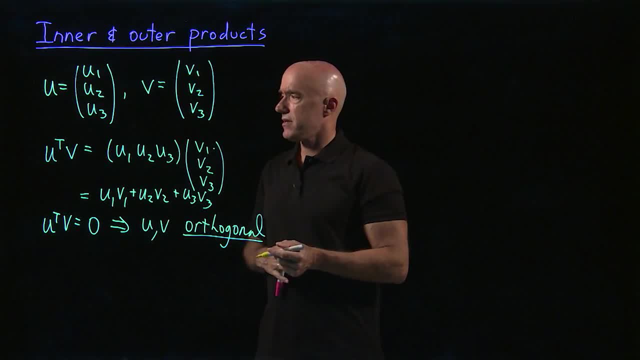 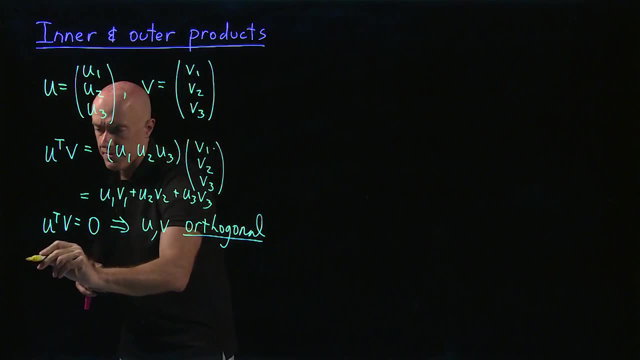 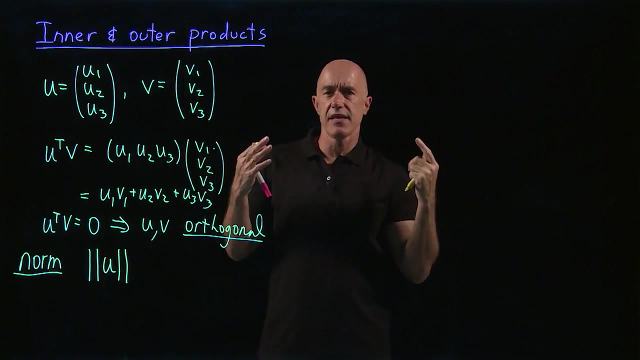 same meaning as perpendicular for the dot product. We have another definition. So we talk about the norm of a vector. This is represented. say, the norm of the vector u is written with these double absolute value signs. You think of this as the length of u. This is given. 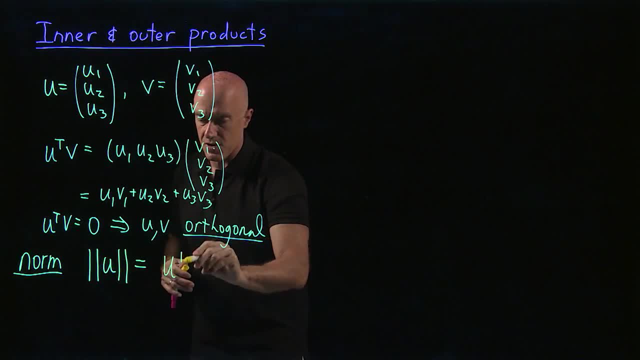 in terms of matrices is u transpose times u. That's a scalar right And we raise it to the 1 half p, Which means taking the square root. So this is just u- u. This is just u 1 squared plus u 2 squared plus u 3 squared. all to the 1 half power or to the square root. Okay, One. 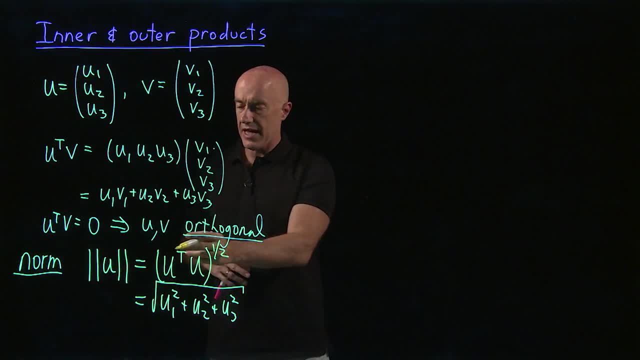 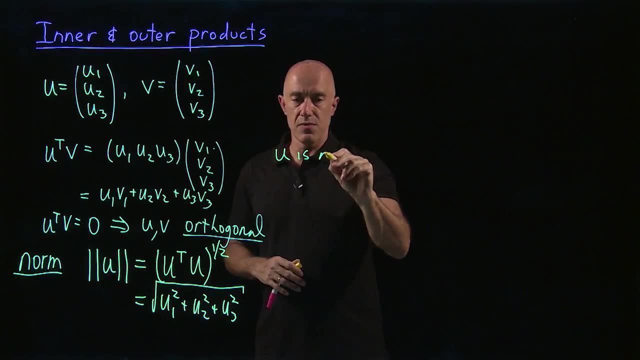 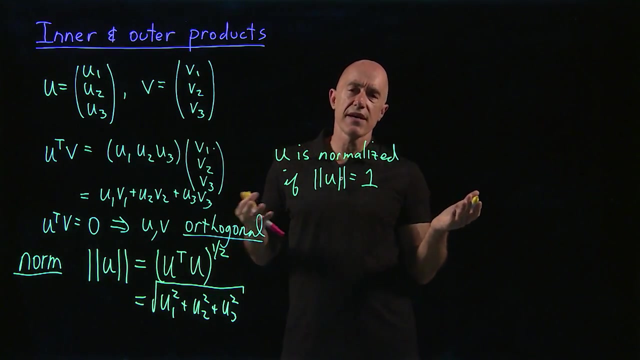 more word we use. We say that u is normalized, So we say u is normalized. So we say u is normalized if the norm of u is equal to 1.. Okay, So we say vectors are normalized if their norms are 1.. So usually you do that: You normalize a vector by dividing by the 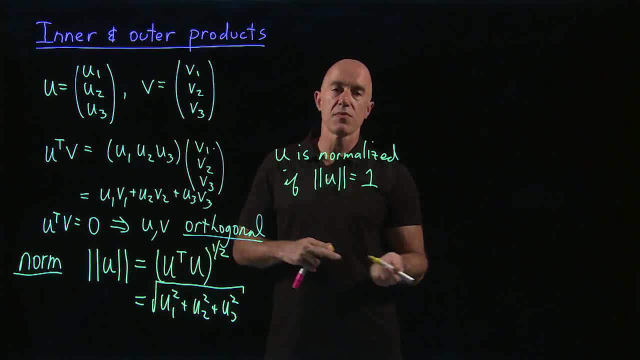 norm of the vector. Okay, Then the vector is normalized. Okay, Then there's another terminology: If two vectors are orthogonal plus normalized, Okay Then. so that means we have two vectors, u and v. They're orthogonal, So u transpose, v equals. 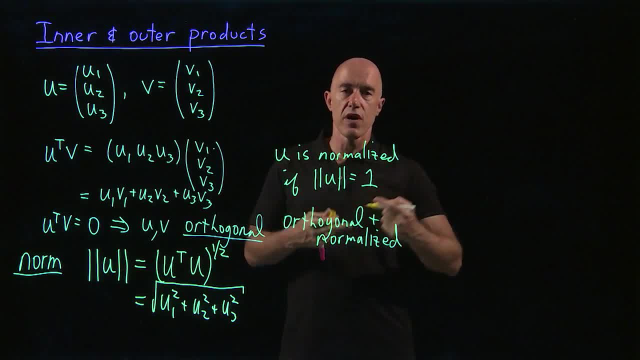 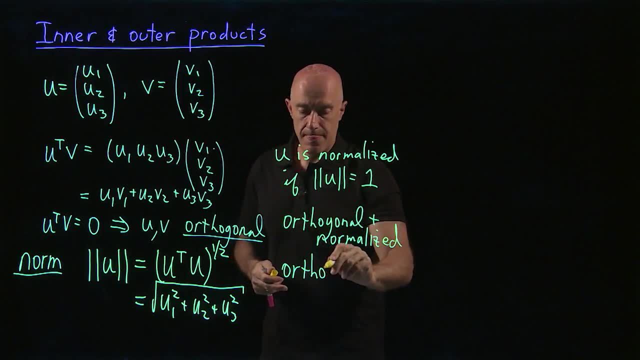 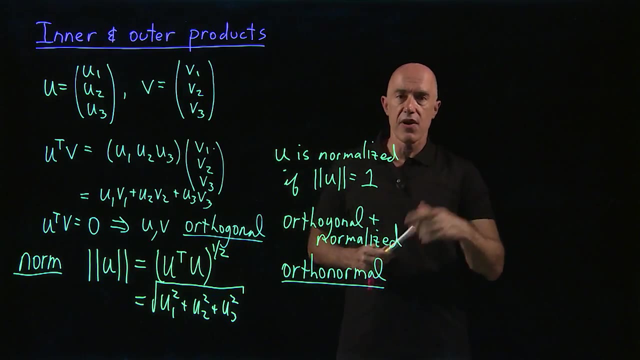 0. And they're normalized. So the norm of u is 1 and the norm of v is 1.. Then we say that the vectors are orthonormal. Okay, So that's a word that is used very frequently in matrix algebra. Okay, So this is all about inner products. Let's see what is the outer. 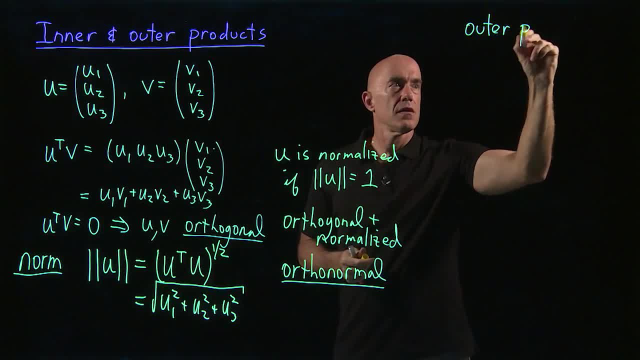 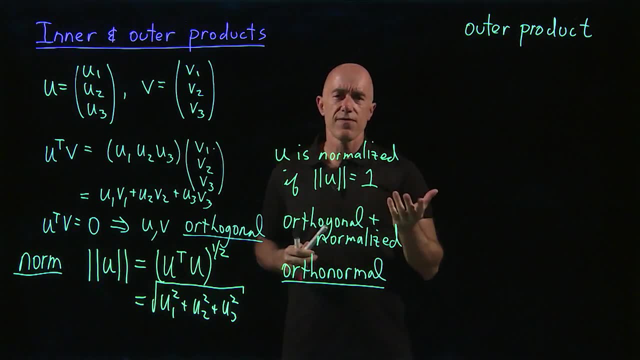 product. The inner product is used all the time. The outer product is not used all the really use that often. but there are some numerical methods, there are some techniques that make use of the outer product. So as a student in matrix algebra, you should know what. 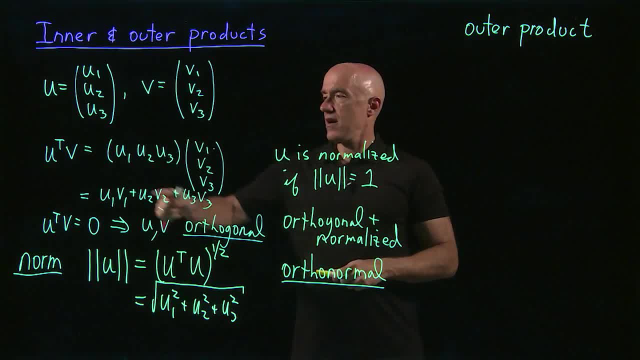 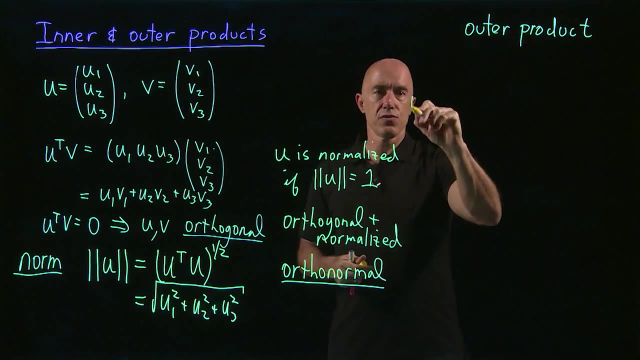 an outer product is The inner product. between two vectors was u transpose v for two column vectors. That gave us a scalar. But what would happen if we did u v transpose? So what would u v transpose look like? So now u is a column vector right, So u1, u2, v3. And v transpose. 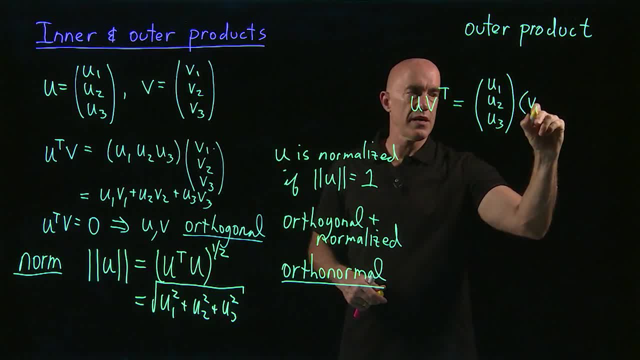 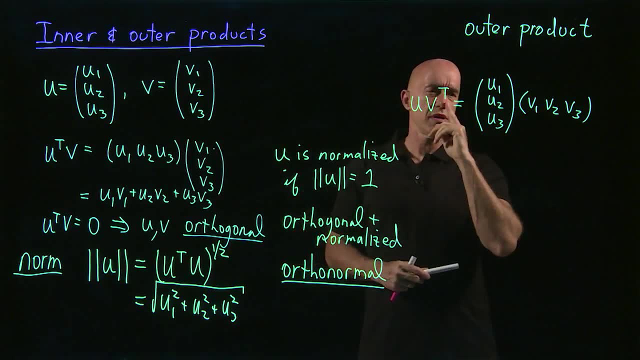 then is a row vector, So that would be v1,, v2,, v3.. So it's this funny multiplication, right? So what is this? This is three by one, right? Three rows, One column, Three by one. This is one by three: One row, three columns, Three by one times. 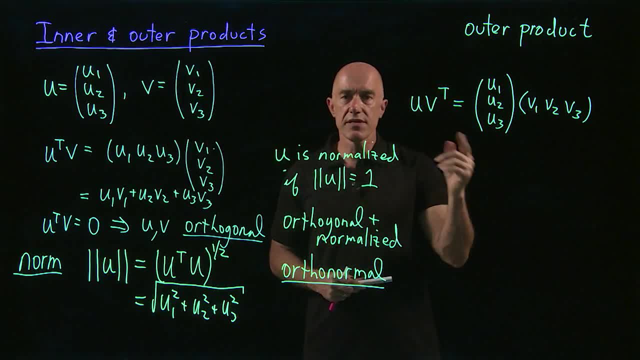 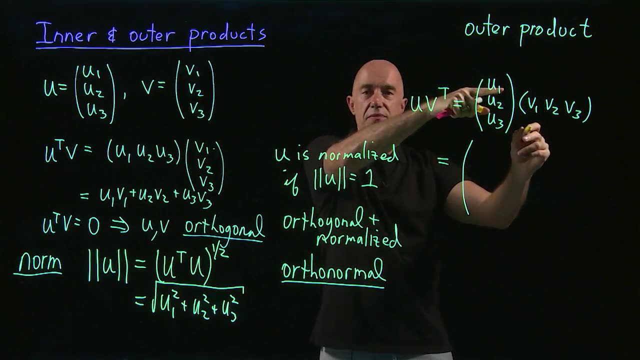 one by three is three by three. So this is a three by three matrix. okay, Rather odd looking. So we can calculate it. So go across the first row down the first column. Kind of boring right. There's only one element in the first row and one element in the first. 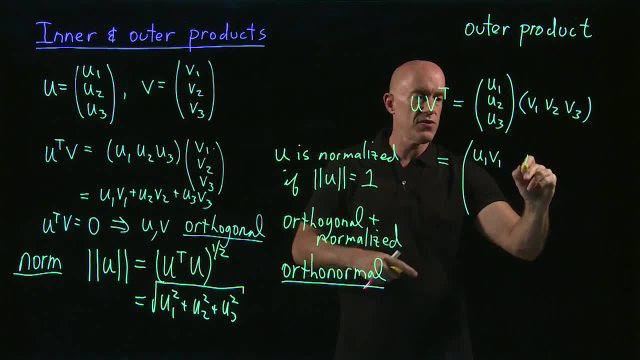 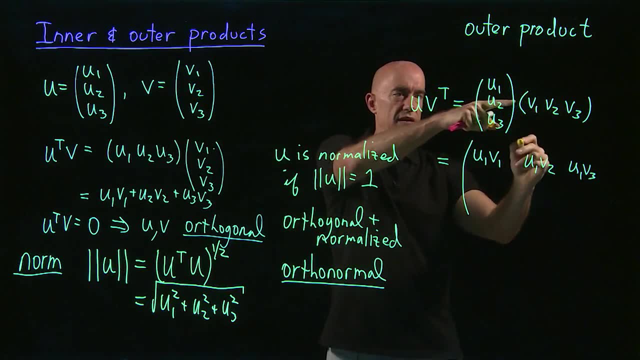 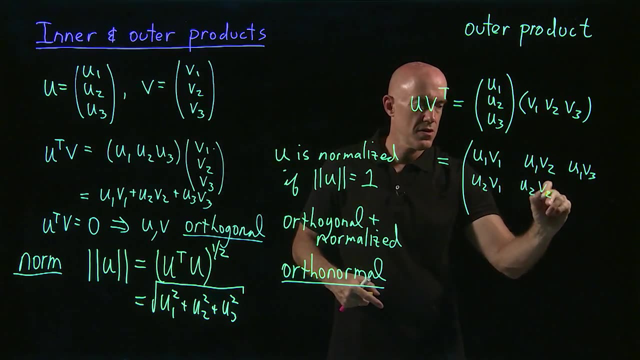 column. So that's u1, v1, u1, v2, u1, v3, right, And then the second row, first column u2, v1, u2, v2, u2, v3.. And then finally u3, v1, u3, v2, u3, v3.. 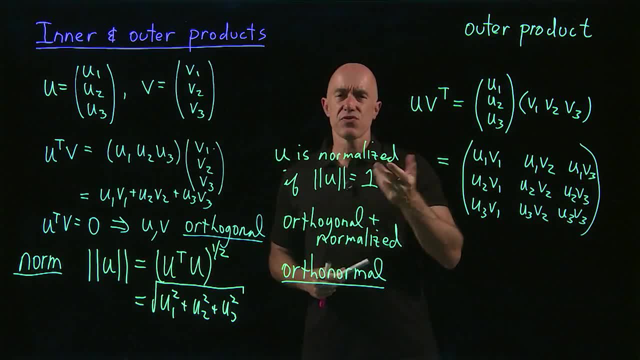 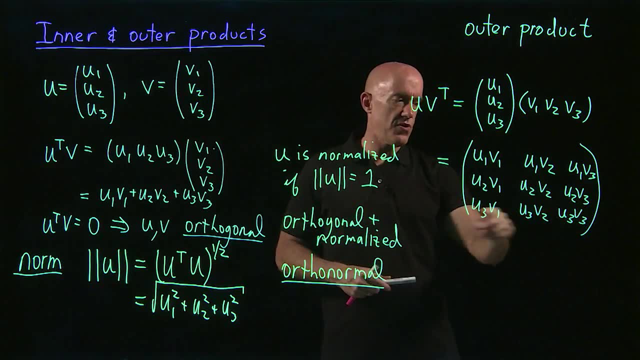 Okay, Three by three matrix. It's a rather strange matrix. The first row has u1, the second row has u2, the third row has u3.. The first column has v1, the first column has v2, the first column has v3.. Well, we'll see that this type of matrix in some sense lives. 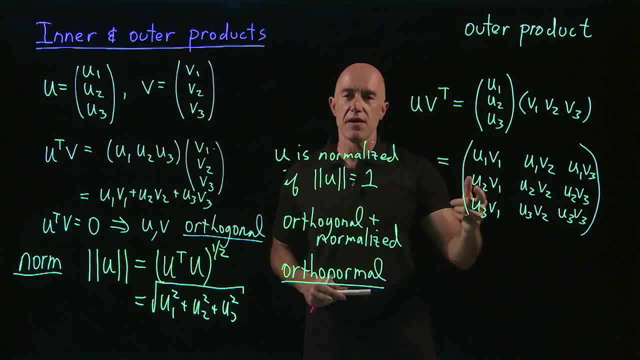 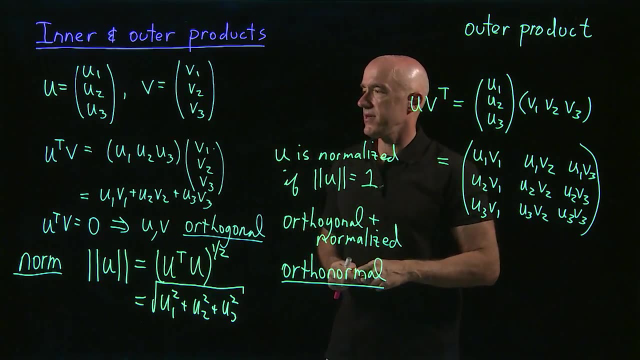 in a very low dimensional space, But we'll talk about that more when we talk about a more advanced topics in matrix algebra. Okay, So let's recap: We're talking about inner and outer product spaces here. So the inner product between two column matrices is a. u transpose v, That gives us a scalar. 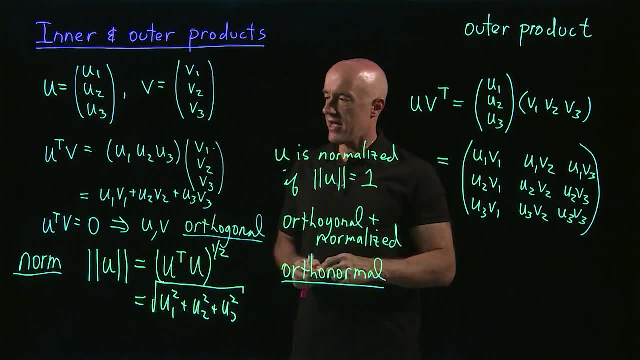 That's equivalent to the dot product. in vector calculus, If u transpose v equals zero, then we say the two vectors are orthogonal. Okay, The norm of the vector, which is equivalent to the length of the vector, is: u transpose u raised to the half power, so square root of the sum of the squares of the components.